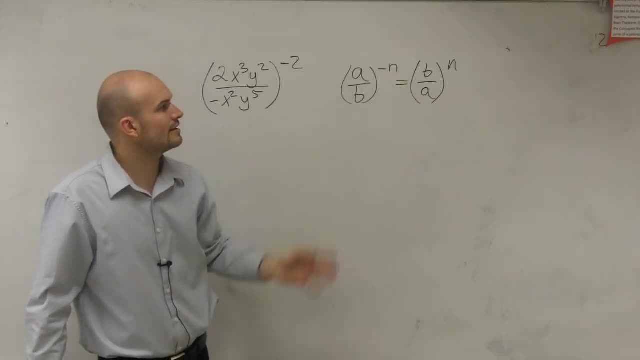 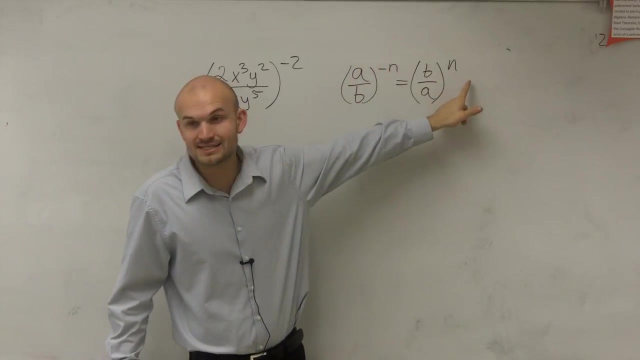 And there's a reason why: because if you put that under one- and you know I can go through the whole explanation, But just so you understand, if you have A divided by B raised to a negative exponent, to make that exponent positive. 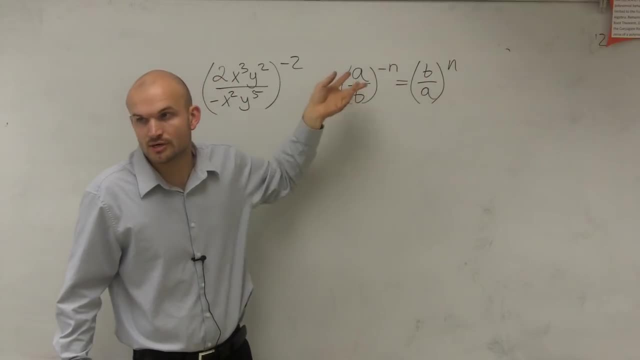 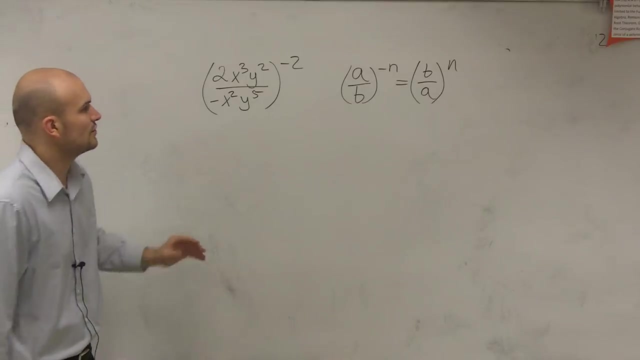 you just need to make sure you're dealing with the reciprocal of your term. Do you guys see how that kind of works? Okay, I'll go through. went through whole explanations already before, so let's just go through this. So therefore, I want to make sure I deal with the positive exponent. Therefore, I need to take the reciprocal of my rational function. 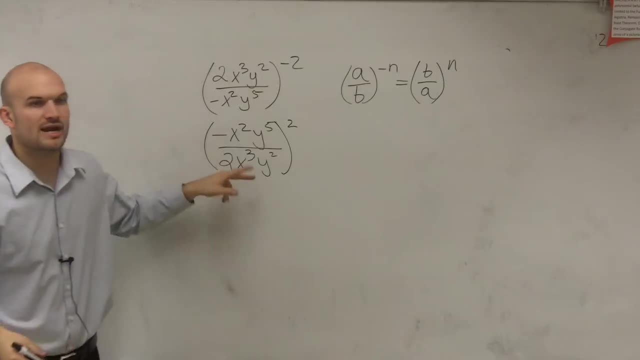 Okay, so then I flip the inside and now I can make that a positive exponent. That's kind of step number one. The second step is the power to product rule. So that's step number one. Second step is power to product rule. 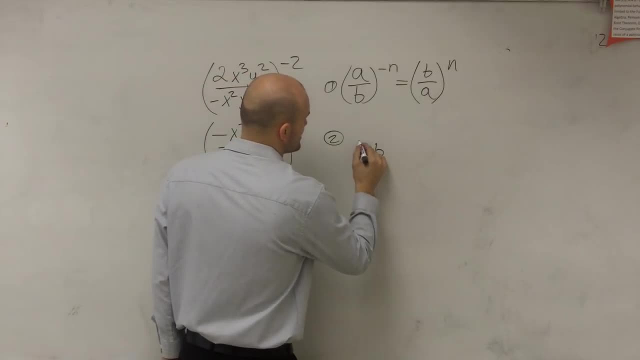 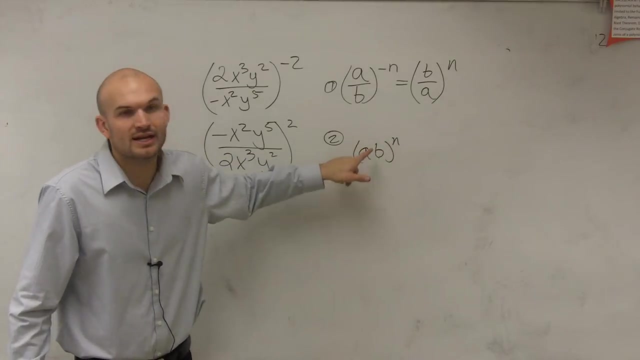 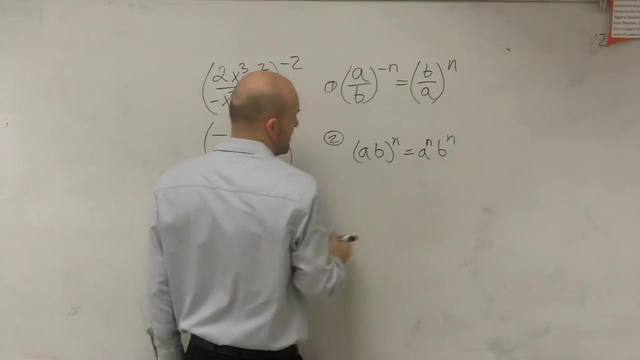 And what the power to product rule says is if I have a product raised to a power, then that power is distributed to both of my terms in the product Meaning And that goes A to the N and B to the N. That also works for my product and my quotient. 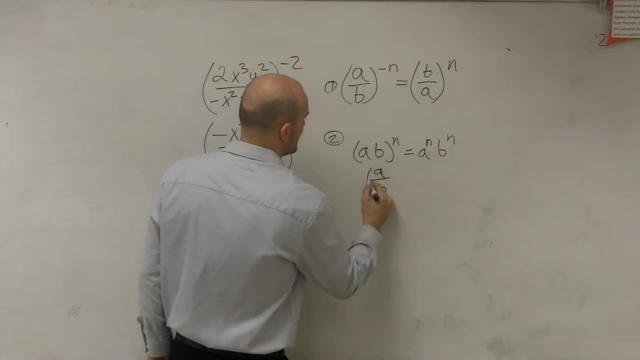 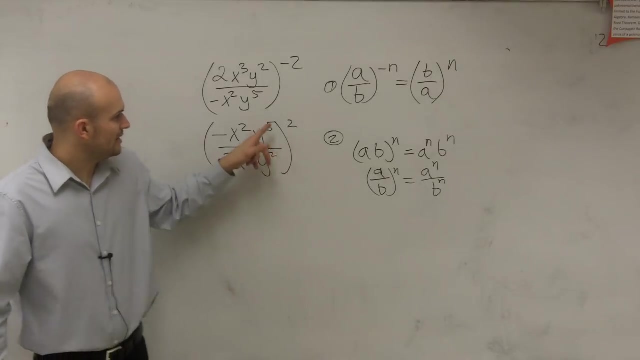 If I have A divided by B raised to the N, that equals A to the N over B to the N. So what this is telling me right now is: everything inside of here needs to be raised to the second power, Everything. So, therefore, what I'm going to do is just rewrite everything to the second power. 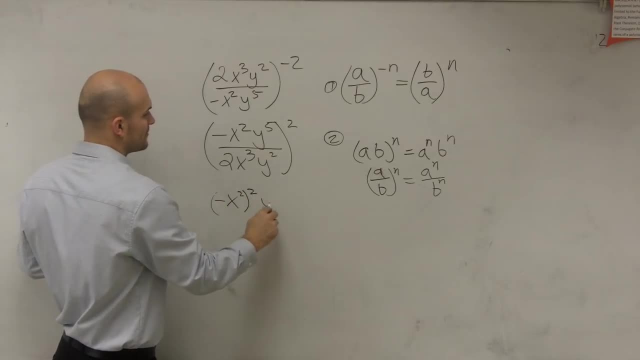 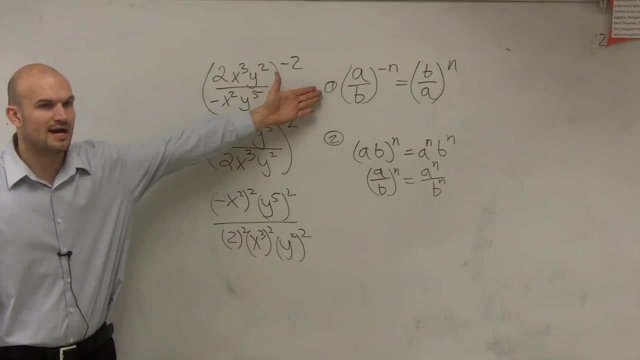 So negative: X squared squared, Y to the fifth squared over 2, squared X cubed squared and Y squared squared. Does everybody see that? So the first thing you apply is being the reciprocal. Then you use the power and quotient of power. 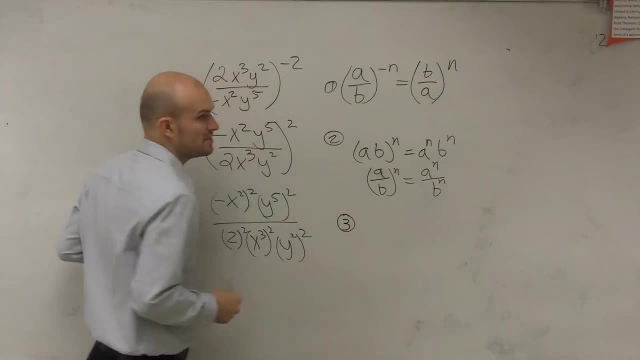 Then the third one is you're going to use the power of power rule Which states: if you have A raised to an exponent raised to an exponent, then that simply means A to the M times N. So now you're going to multiply the two powers. 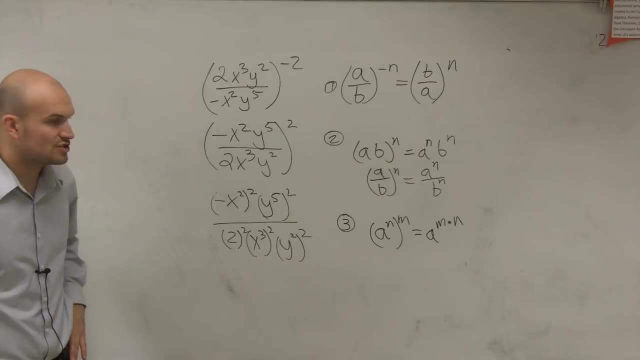 So on my final step, I'll have negative X squared squared. So negative X squared times negative X squared is now going to be a positive X to the fourth. Then I have Y to the 10th divided by 4, X to the 6th, Y to the 4th.